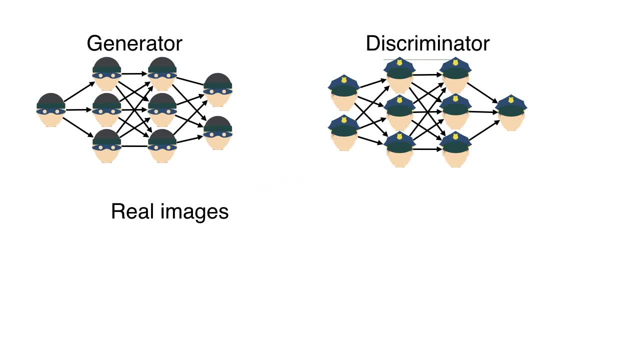 of fake images generated by the generator. The discriminator is trained to identify which images are real or which ones come from the generator, and the generator is trained to fool the discriminator into classifying its images as real images. In this video, we will build a very, very simple pair of GANs. 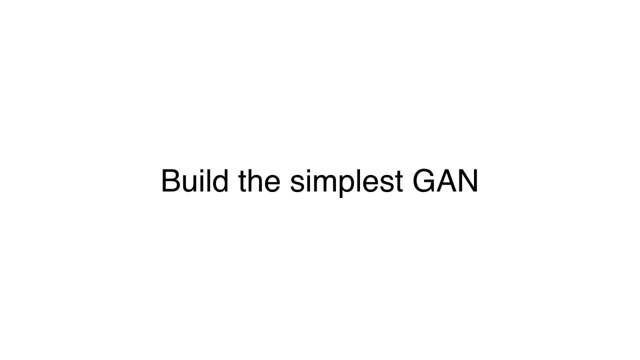 so simple that we'll be able to code them straight in Python without any deep learning packages. This is our setting. We live in a world called slanted land, where everybody looks slightly elongated and walks at a 45 degree angle. This world has 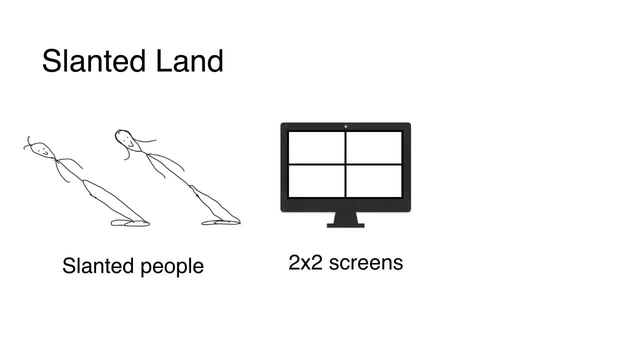 technology, but not as developed as ours. They have computer screens which display images, but the best resolution they've been able to work out is 2 times 2. So they have black and white, two pixels by two pixel screens. Also, they have developed neural networks, but only very simple. 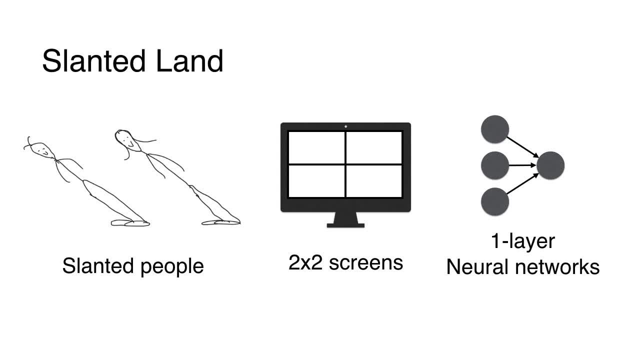 ones. As a matter of fact, they only know neural networks of one layer, But I will show you that in this simple world, we can still create a pair of GANs that will generate faces of the people who live in slanted land. 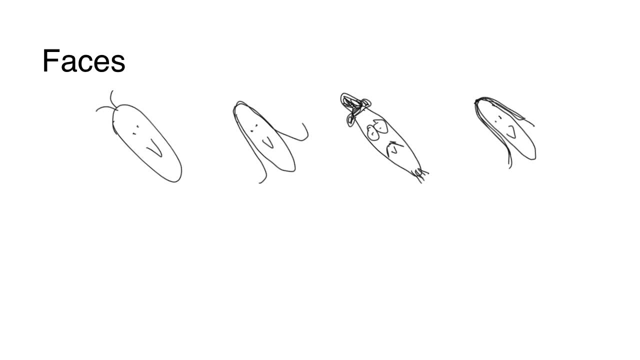 Here are four faces of people who live in slanted land. Notice that everybody is elongated and tilted 45 degrees to the left, Since the screens are only 2 pixels by 2 pixels. this is how the pictures of the people look in the screen. 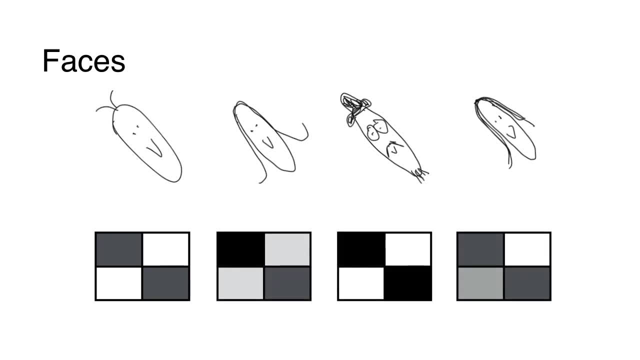 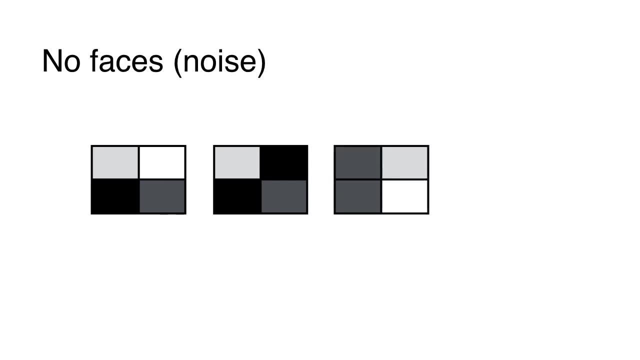 They mostly look like a diagonal or a backwards slash, and this is how noisy images look. Notice that these are not faces, since they don't look like a backlash and these are mostly generated randomly. So the goal of our networks is to be able to distinguish faces. 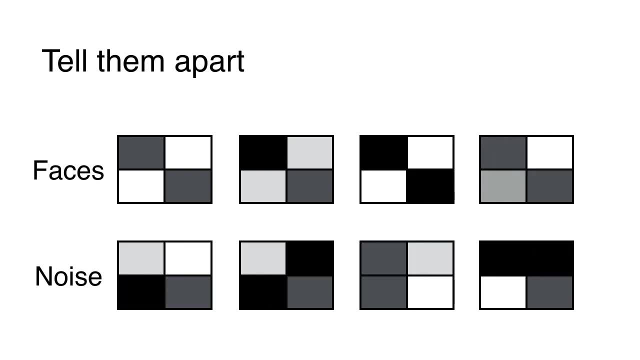 like these, from noisy images like these. Let's attach some numbers here. We'll have a scale where a white pixel has value 0 and a black pixel has a value of 1.. You may have seen this in the opposite way, but we'll do. 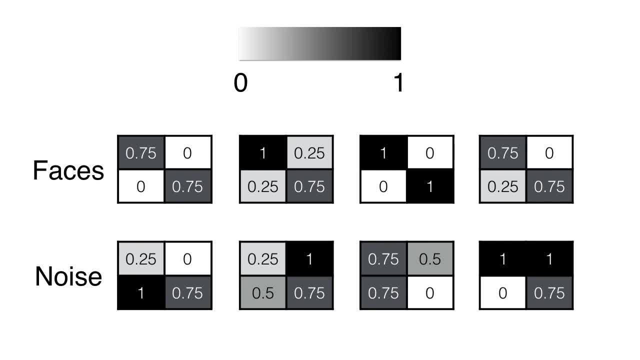 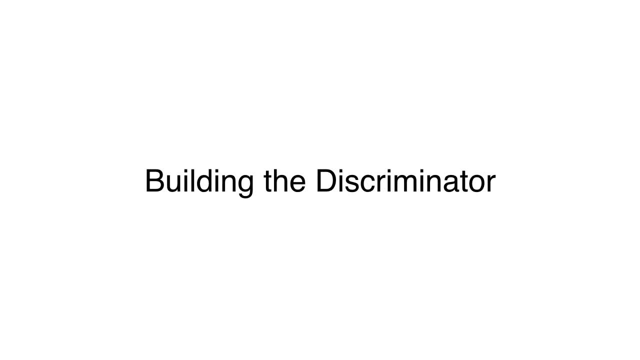 it like this for clarity: This way, we can attach a value to every pixel in the 2x2 screens. Okay, we're ready to build our networks. First I'll build them by hand, and then I'll show you how to get the computer to train them. Let's start by building the discriminator. 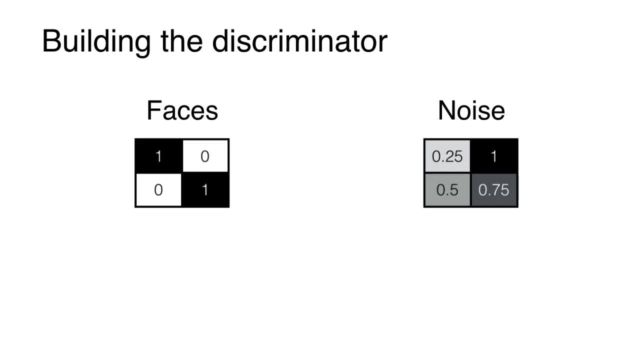 The first question is: how are we going to tell faces, apart from non-faces, Easy? Notice that in the faces, the top left and the bottom right corners have large values because their pixels are dark, whereas the other two corners have small values because their pixels are. 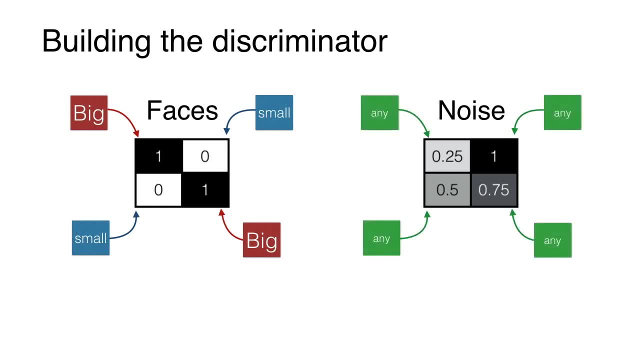 light. On the other hand, in noisy images, anything can happen. Therefore, the way to tell faces apart is by adding the two values corresponding to the top left and bottom right corners and subtracting the values corresponding to the bottom left and bottom right corners. 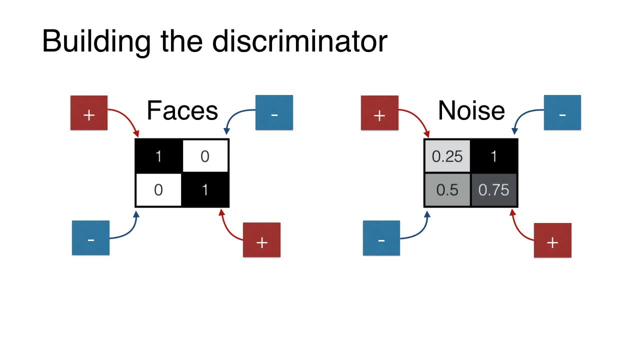 In faces, this result will be very high, whereas in noisy images it will be low. For example, for this face, the value is 2, and the value for the noisy image is minus 0.5.. We can add a cutoff or a threshold of, say, 1, and say that any image that scores 1 or higher is. 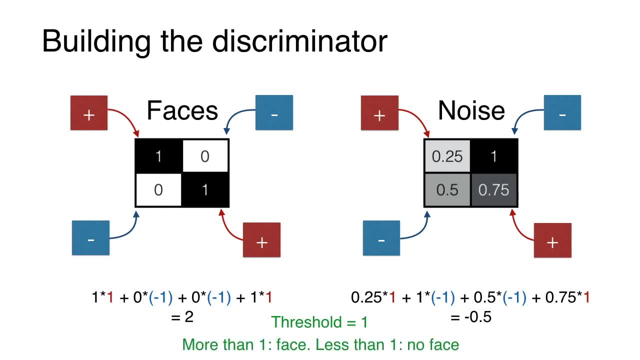 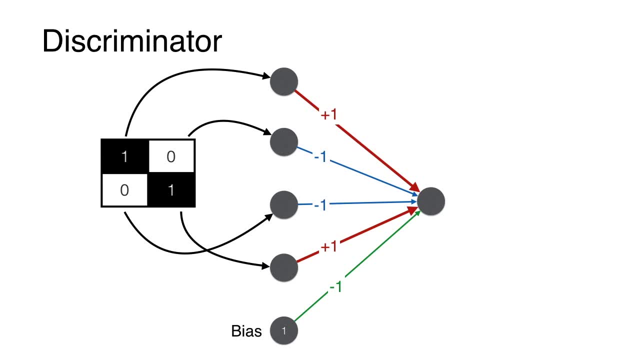 a face, and any image which scores less than 1 is not a face or is a noisy image In neural network lingo. this is how things look: The values of our four pixels get multiplied by plus or minus 1, depending on what diagonal they are on, and then we subtract the total. 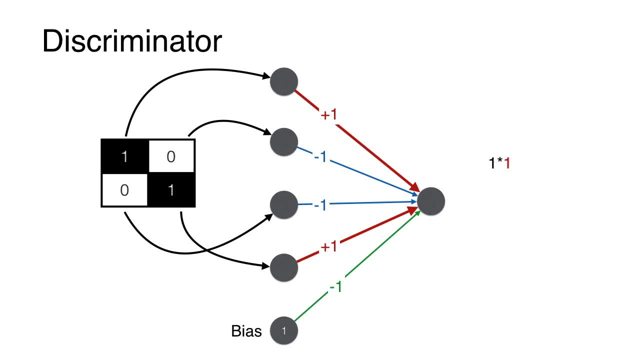 value of 1, or the bias. We add these four numbers and if the score is 1 or more, then the image is classified as a face, and if it's less than 1, then it is classified as not a face. In this case, the image is a face because it gets a score of 1.. 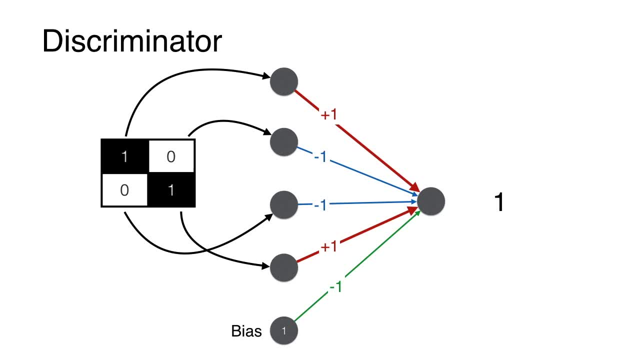 We can also output the probability that something is a face by using the sigmoid function. We apply the sigmoid, which is this function that sends high numbers to numbers close to 1, and low numbers to numbers close to 0, and we get sigmoid of 1, which is 0.73.. This. 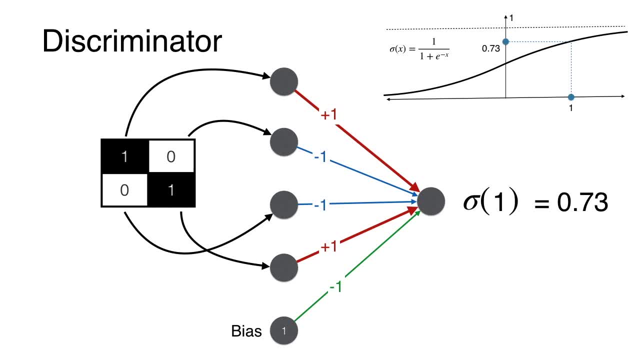 discriminator network then assigns to this image a probability of 73% that it is a face. Since it is a high probability, greater than 50%, we conclude that this discriminator network thinks that the image is a face, which is correct. Notice that in this neural network, 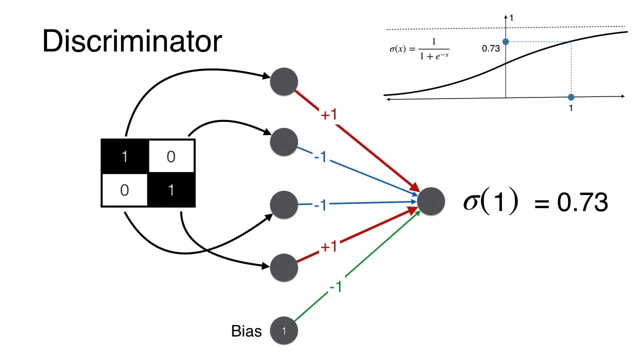 the thick edges are positive and the thin ones are negative, and this is a convention we'll be using throughout this video. Now, if we enter the second image, which is not a face, into a discriminator, then we do the same calculation and we get negative 0.5 for the score Sigmoid of negative 0.5. 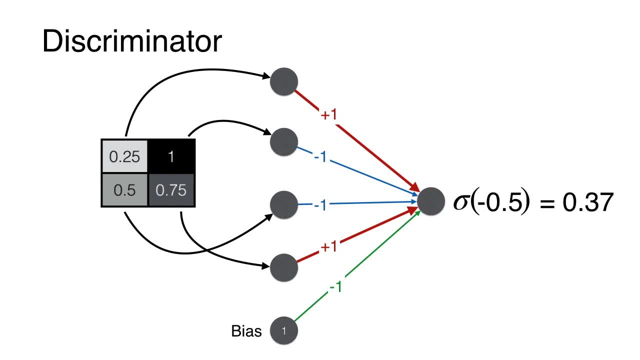 is 0.37. This is lower than 50%. so we can get a score of 0.37, which is 0.37.. This is lower than 50%. so we conclude that this discriminator network thinks that the image is a face. 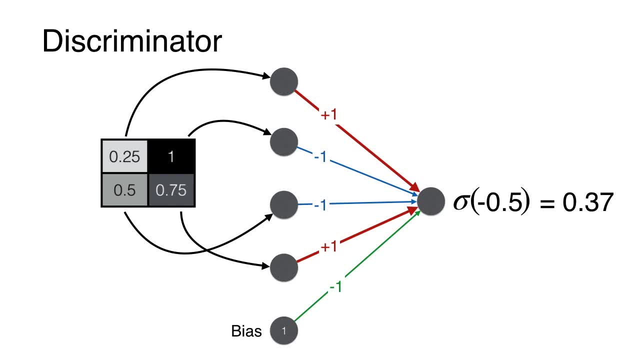 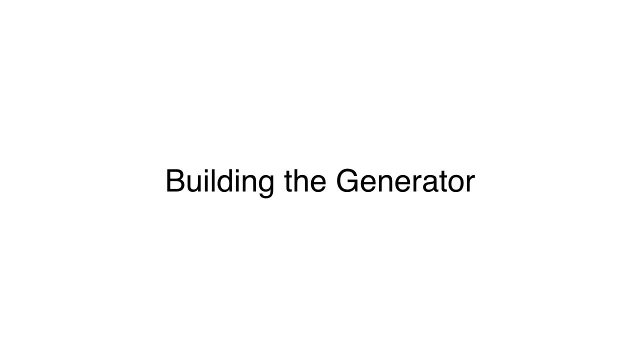 which is not a face. The discriminator is correct again. Now, in the same way, let's build a generator. This is a neural network that will output faces To build a generator. we'll again take into account that among faces, these two corners, 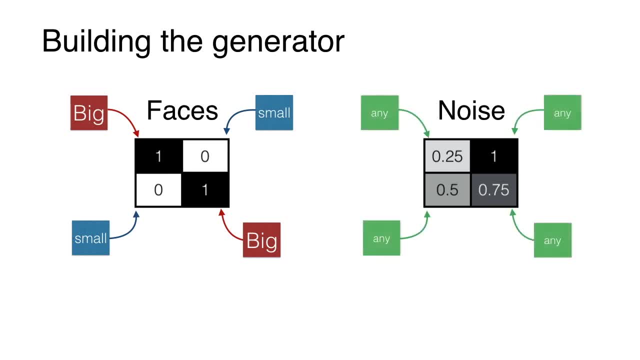 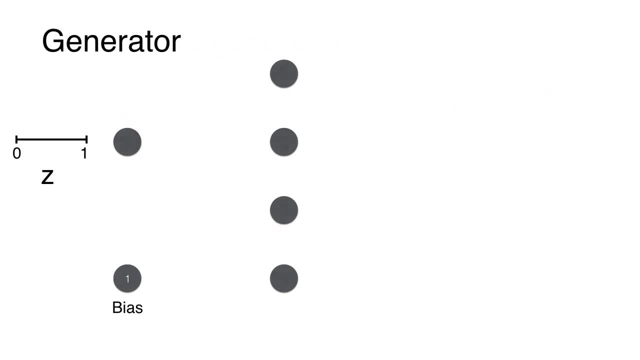 are high value. these two corners are low value, whereas in noisy images or non-faces, anything can happen. So this is how the generator works. First, we start by picking an input, z, which is a random number between z and 0.. 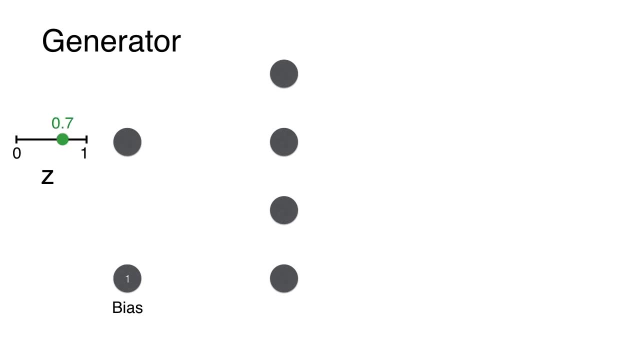 In this case, let's say it will be 0.7.. In general, the input would be a vector that comes from some fixed distribution. Now let's build a neural network. What we really want is to have some large values and some small ones. The large ones are represented by thick edges and the small ones by thin. 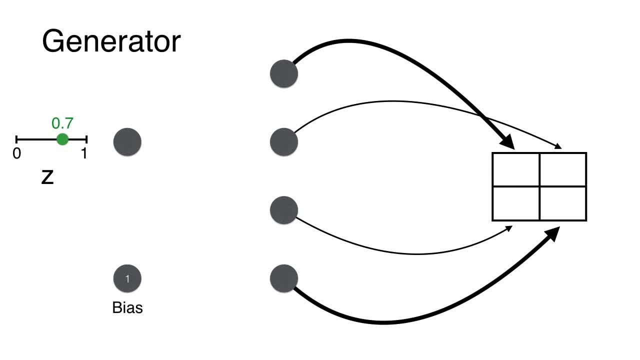 edges, Because remember that we want large values for the top left and bottom right corner and small values for the top right and bottom left corner. So since the top output has to be large, we want these weights coming in to be large, so let's make them plus ones. 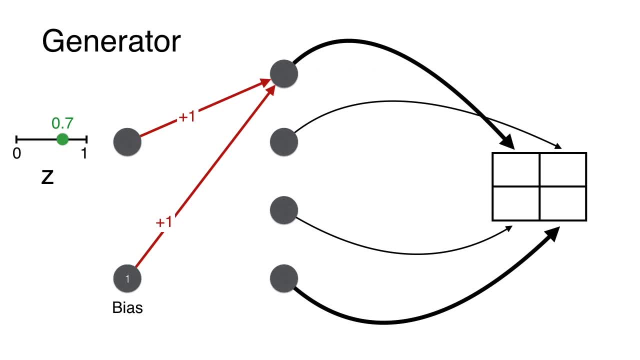 Now, what do we get for the output here? Well, first we're going to get a score of plus one times 0.7, plus one which is 1.7.. Now let's look at the second node. It corresponds to the top right corner, so it has to be a. 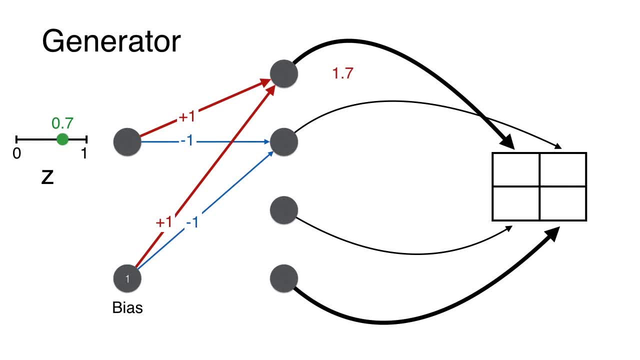 small value, So let's put negative numbers here. What do we get for the score? We get minus one times 0.7, minus one times 0.7. And we get minus one times 0.7, minus one times 1, which is minus 1.7.. In the same way, we want a small value here, so we put 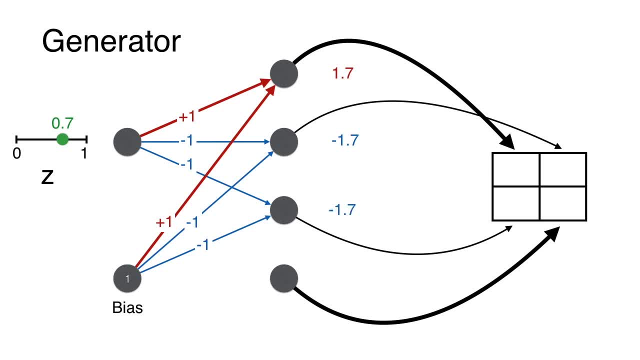 weights of minus one and we get minus 1.7. And for the last one we want a higher value. so we put plus ones and we get plus one times 0.7, plus one, which is 1.7.. 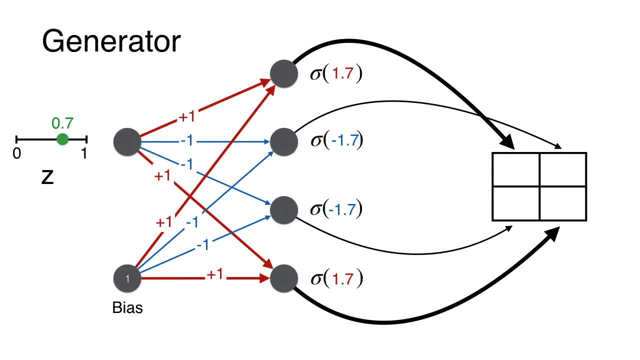 Now, those are just the scores. We need to apply sigmoid to find the probabilities. So we apply sigmoid and we get 0.85, 0.15, 0.15, and 0.85.. Those are the values that will go in our pixels And notice that our image looks like. 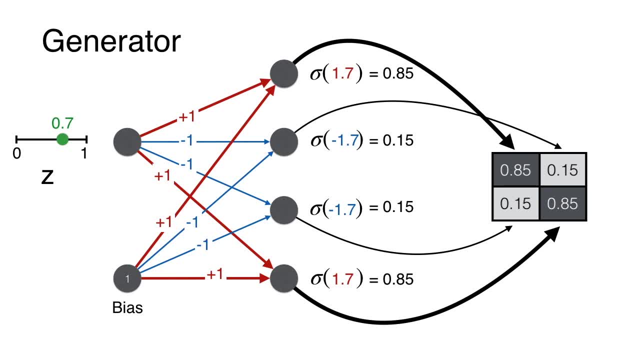 a diagonal, which is how we define our faces. Notice that, by the way we built it, this neural network will always generate large values for the top, left and bottom right corners and small values for the top right and bottom left corners. no matter what values that we 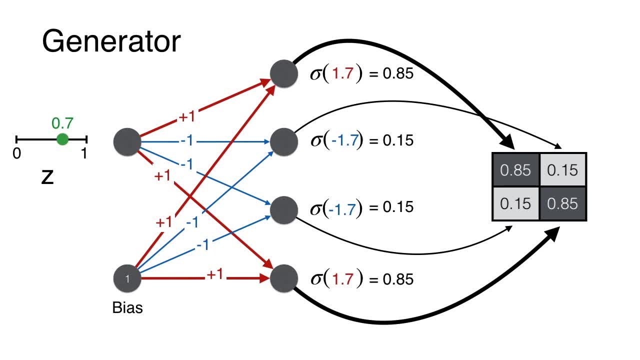 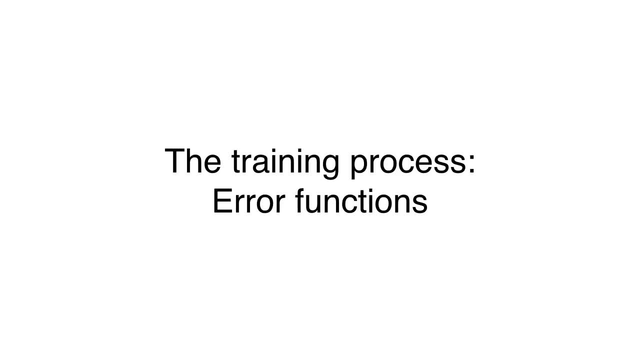 input Because, remember, that is between 0 and 1.. Therefore, this neural network will always generate a face. That means it's a good generator. Of course, we built these neural networks by eyeballing the weights, but that's not. 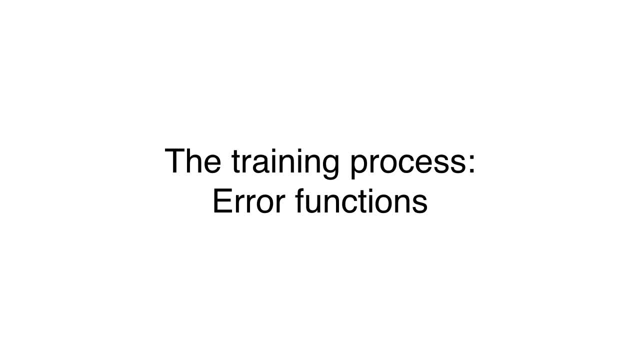 how it's normally done. In general, we have to train the neural networks to get the best possible weights For this. let me tell you a little bit about error functions. An error or cost function is a way to tell the network how it's doing in order for it to improve. 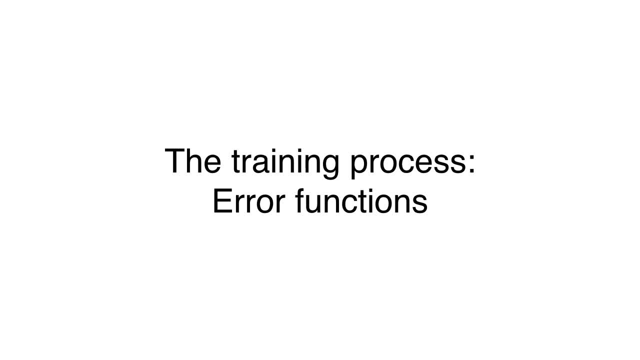 If the error is large, then the network's not doing well and it needs to reduce the error to improve. The error function that we'll use to train these gallons is the log loss, which is the natural logarithm. This is the logarithm basis. 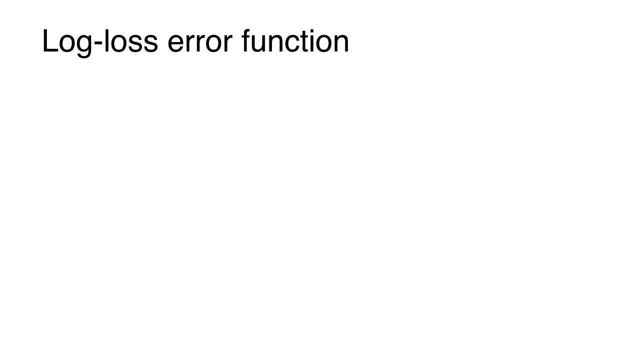 It's E. Why the logarithm? Well, logarithm appears a lot in error functions for many deeper reasons which we will not cover, but we can think of it for now as a very convenient function. Let's first say that we have a label of 1, and our neural network predicted this as 0.1.. 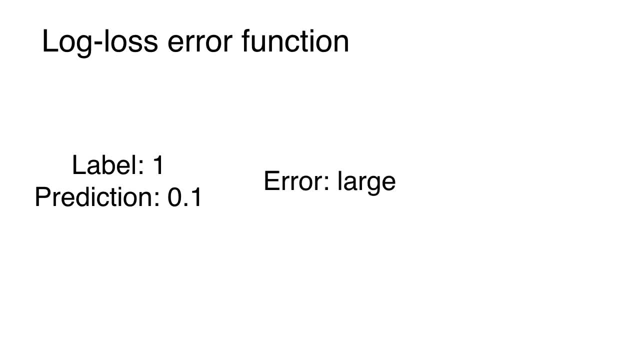 This is a bad prediction and we should produce a large error, because 0.1 is very far from 1.. On the other hand, if the label is 1, and the prediction is 0.9,, then that's a good. 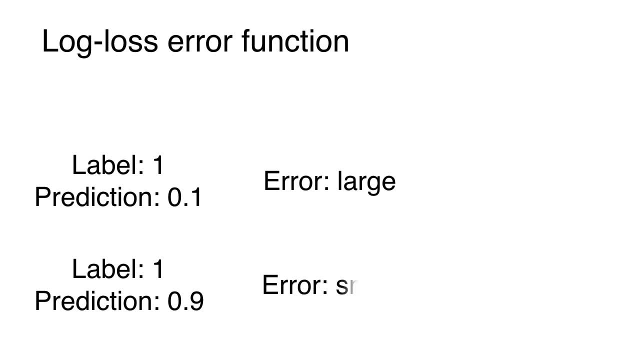 prediction. The prediction is very close to the label, so this should produce a small error. How, then, can we find a formula for this error? Well, notice that the negative natural logarithm of 0.1 is 2.3,, which is large, while the negative 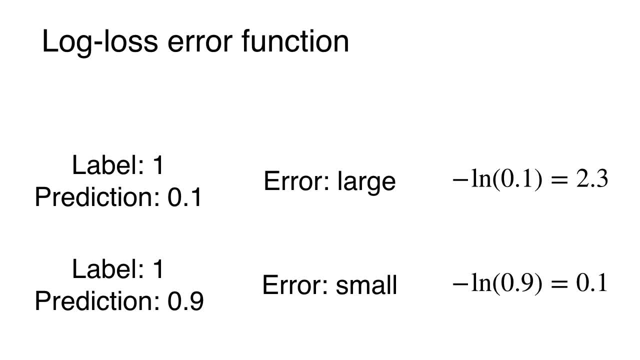 logarithm of 0.9 is 0.1,, which is low. As a matter of fact, the closer a number is to 1,, the smaller its negative logarithm gets. Therefore, when the label is 1,, the function negative logarithm of the prediction is a good. 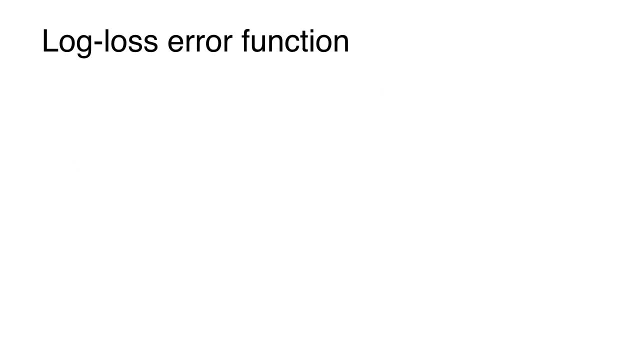 error function. Now let's go in the other extreme, when the label is 0.. In this case, if we had a prediction of 0.1, it would be good because it's close to the label. Therefore, the error should be small. 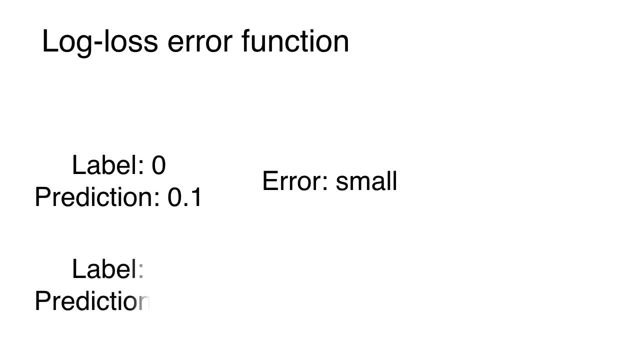 On the other hand, a prediction of 0.9 is terrible, so the error should be large. The function that we need here is similar to the previous one. It is the negative logarithm of 1 minus the prediction. Notice that in the first case, the error is the negative logarithm of 0.9, which is 0.1,. 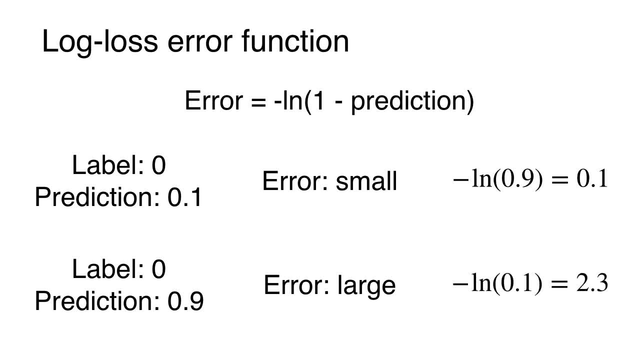 and in the second case, it's the negative logarithm of 0.1,, which is 2.3.. And this matches what we wanted, which is that the first error is small and the second is large. To summarize, if the label is 1,, which means we want the prediction to be 1,, we define. 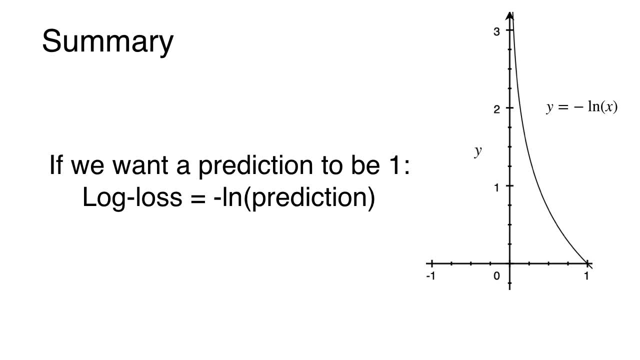 the log loss to be negative. logarithm of the prediction. Notice that from the graph of negative logarithm of x on the right. this is big when the prediction is close to 0, and small when the prediction is close to 1.. And then when the label is 0,, which means we want the prediction to be close to 0 then 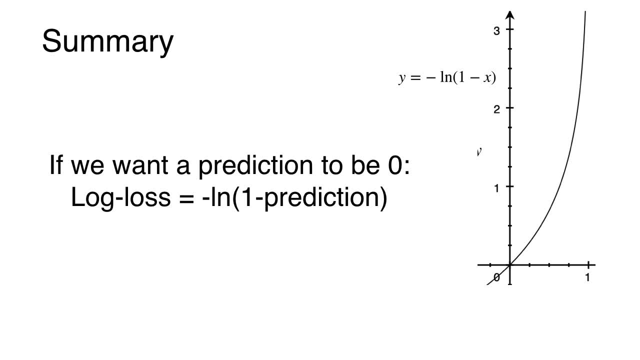 we use as an error function the negative logarithm of 1 minus the prediction, minus x. in the right we see that when the prediction is close to zero, there's a low error and when the prediction is close to one, there is a high error. So these two are the error functions. 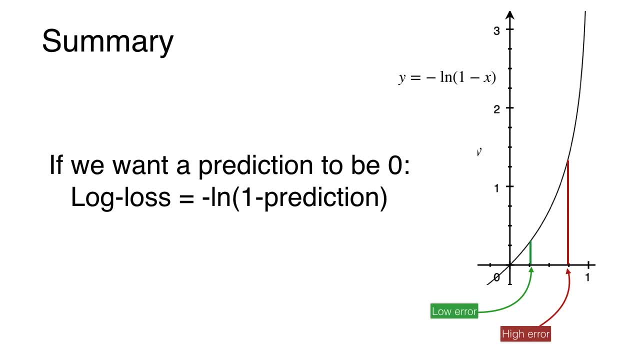 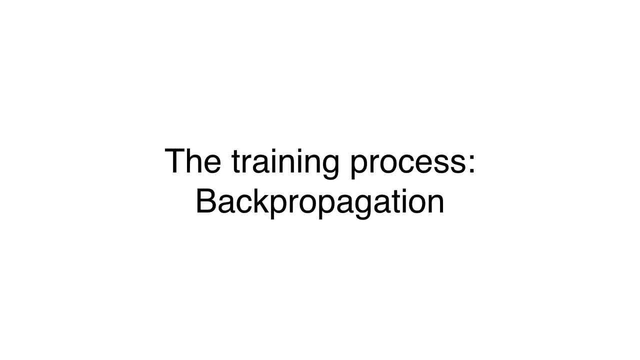 that we're going to use for training: the generator and the discriminator based on if we want the prediction to be zero or one. Now that we have our functions, we get to the meat of our training process, which is back propagation. I will explain it very briefly. The way we train a neural 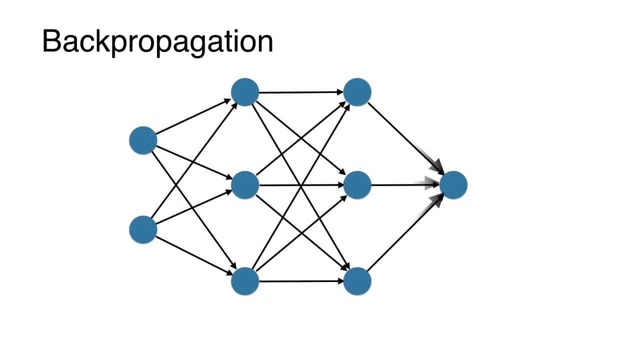 networks by first taking a data point and performing a forward pass, calculating the prediction and then calculating the error based on the log loss that we previously defined. Then we proceed to take the derivative of the error based on all the weights using the chain rule. This will tell us how much to update each weight in order to best decrease the error. The 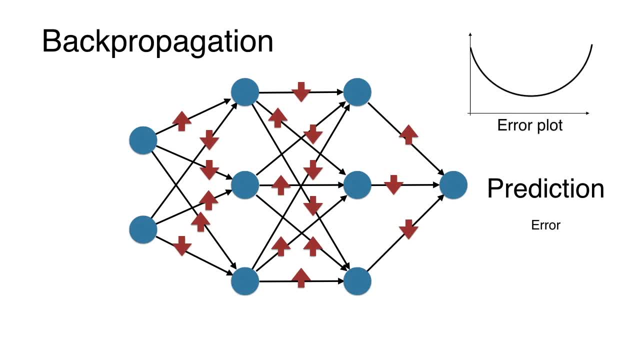 way we do the error using a derivative is a process called gradient descent. Long story short, what you do is you plot the error with respect to the parameters and calculate the gradient which is the direction of greatest growth, and then take a tiny step in the direction of the negative of this gradient. 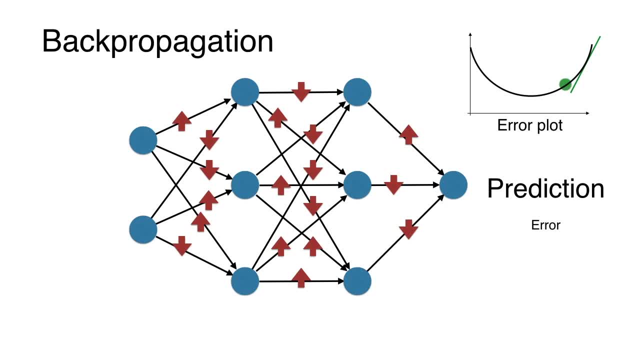 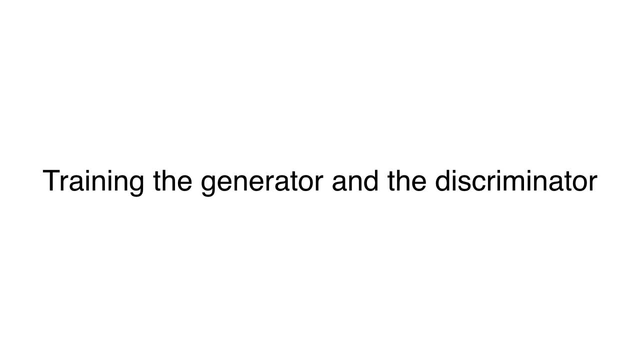 in order to find new parameters that decrease this error as much as possible. Now we're ready to train the generator and the discriminator, and what we have to do is put the right error functions on the right places. Here is our pair of neural networks, and notice that the weights are. 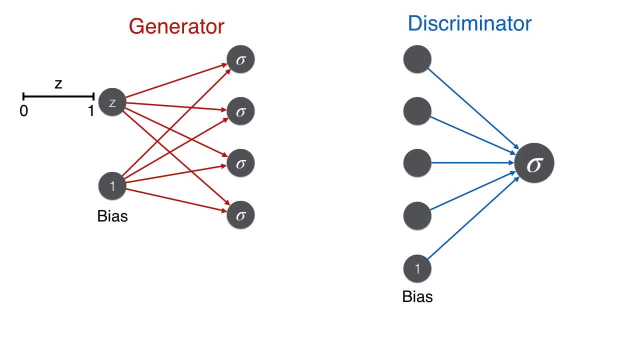 not yet defined. so we start by defining them as random numbers. Now we select, set as some random number between zero and one which is going to serve as the input to the generator. We do a forward pass on the generator to obtain some image which is probably. 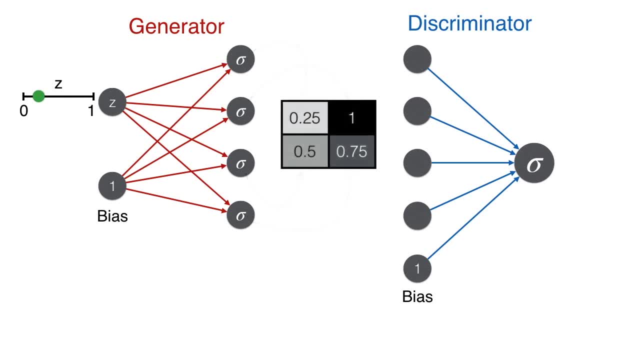 not a face, since the weights are random. This is going to be our generated image. Now we pass that generated image through the discriminator, so the discriminator can tell if it's fake or not. The discriminator outputs a probability, so let's say that it's, for example, 0.68.. Now pay close attention, because this is where the rubber meets the rope. 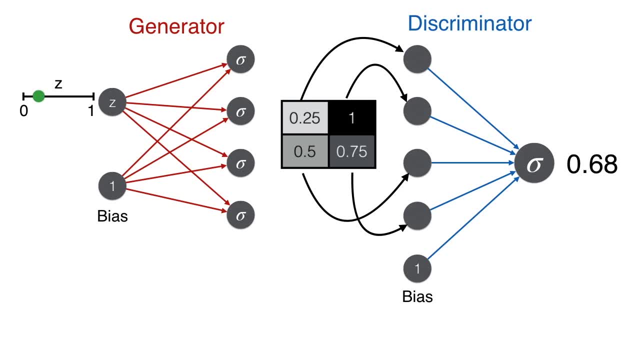 This is where we define the correct error functions. First, let's think: What does the discriminator want to do here? In other words, if the discriminator was great, what should it output? Well, since the image is not a face, but it's a generated image from the generator, then the 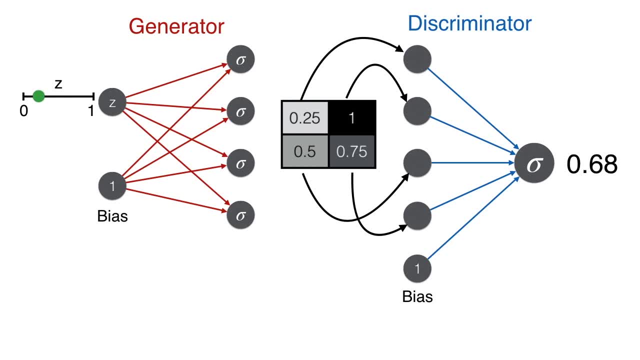 discriminator should be saying that it's fake. That means that the discriminator should be outputting a zero. If we remember the error function, the way we measure an error when we want the neural network to output a zero is the negative logarithm of 1 minus the. 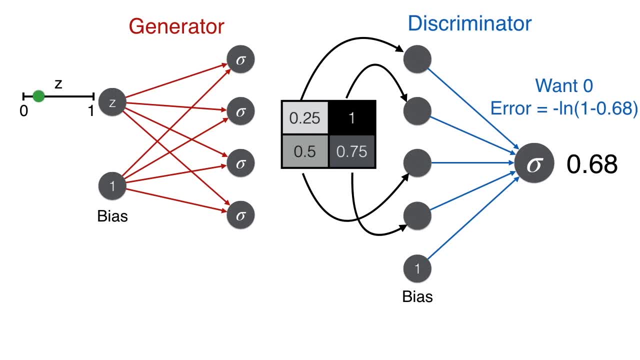 prediction. This is an error that will help us train the discriminator. Now that we've figured out what the discriminator wants, let's go to the generator. What does the generator want? Well, the generator is wildest dream. The generator actually wants to generate. 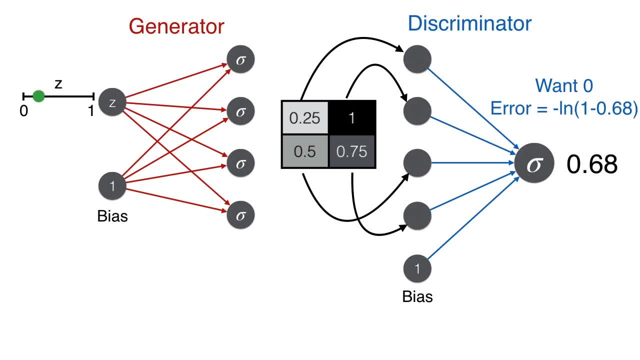 an image so good, so real that the discriminator classifies it as real. Therefore, the generator wants this whole neural network, the connection of the two, to output a one. That means that the error function from the generator is negative logarithm of the prediction. So that is the 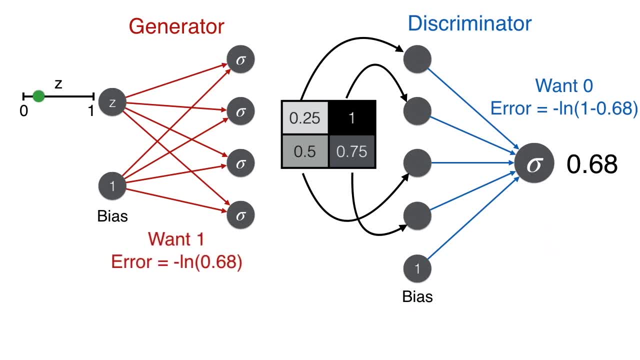 error function that will help us train the weights of the generator. In other words, if, If g of z is the output of the generator and d of g of z is the output of the discriminator, then the error function for the generator is negative. logarithm of d of g of z. 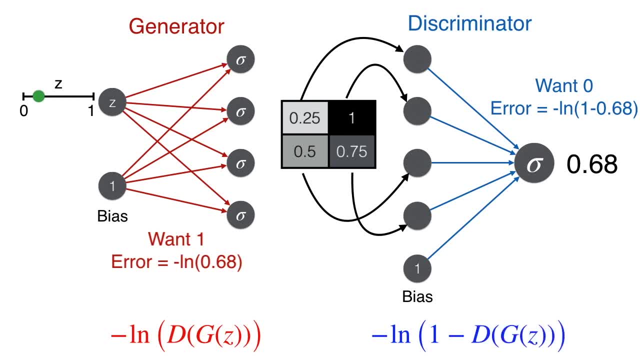 and the error function from the discriminator is negative. logarithm of one minus d, of g, of z. The derivatives of these two are what will help us update the weights of both neural networks in order to improve that particular prediction. Notice that these two error functions. 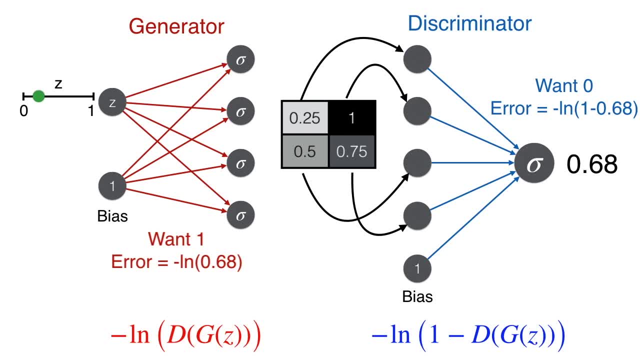 fight against each other. but that is okay, because the red error function only changes the generator weights and the blue error function only changes the discriminator weights. therefore they don't collide. They simply improve both neural networks as one to produce different outputs, which is fascinating. 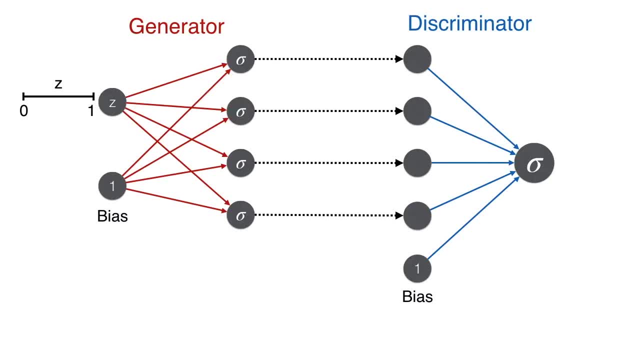 So what we have to do now is repeat this process many times. We pick a random value for z, we apply the generator to produce a fake image, apply the discriminator to that image and use backpropagation to update the weights on both the generator and the discriminator. 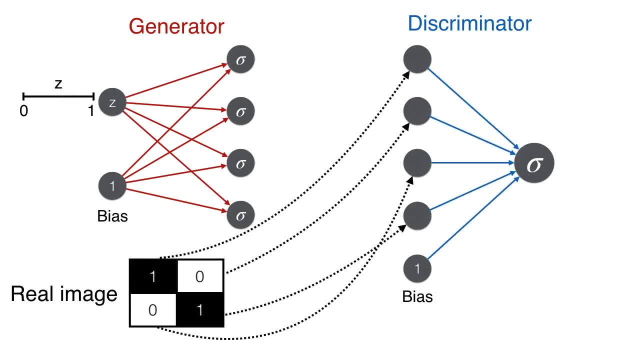 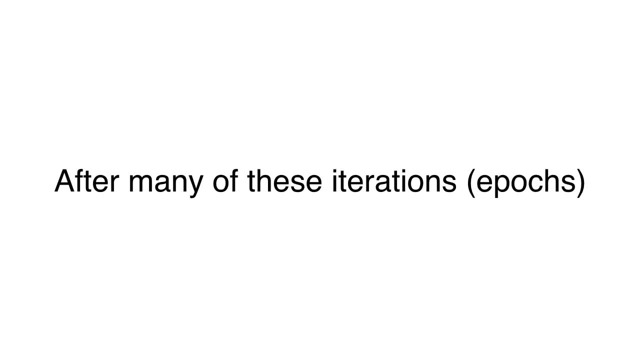 Then we take a real image, plug it into the discriminator and update its weights again using backpropagation. So what happens after many of these iterations or epochs? Well, we left the training in the notebook and we got these values for the weights. 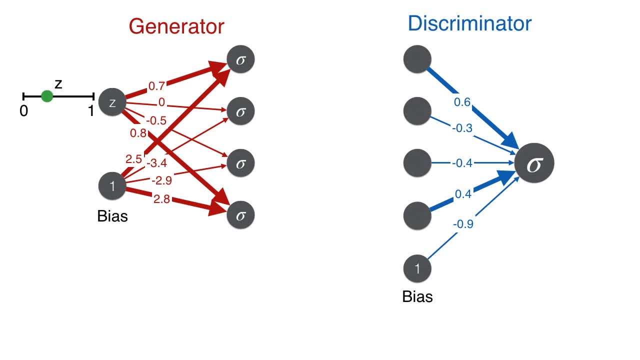 To make it easier, I've drawn thick edges for the positive weights and thin edges for the weights that are negative or zero. Feel free to pause the video and convince yourself that these two neural networks actually work really well, both the generator for generating realistic looking faces. 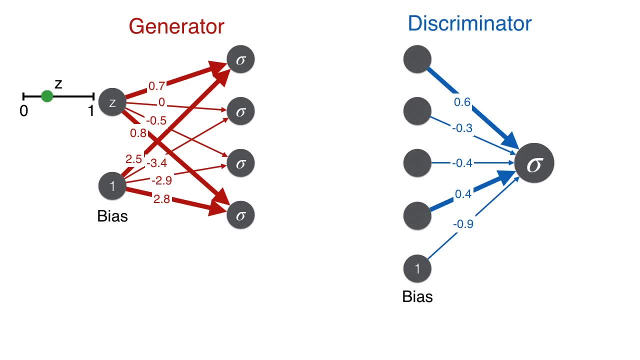 and the discriminator for being able to tell apart the faces from the non-faces. And the reason for this is that, if we remember from the beginning of the video, the top left and bottom right corners of a face should be big and the other two should be small. 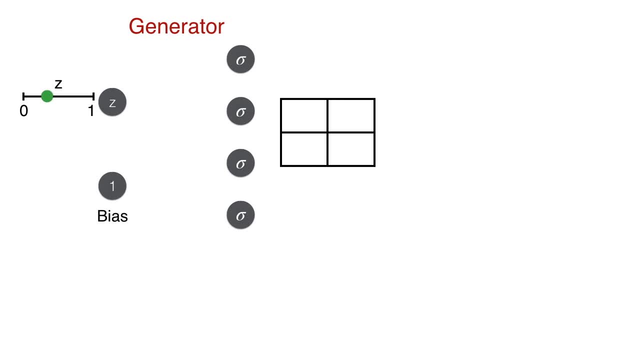 So let's just convince ourselves. Let's look at the generator. Notice that since the input is between zero and one and the two top edges are positive, then the sigmoid value of this output is large, which is the value of this pixel over here. 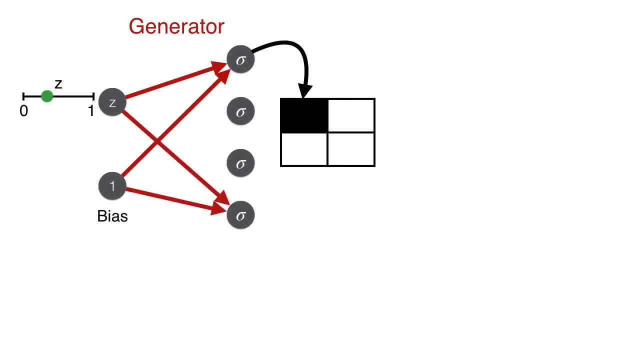 Therefore, that pixel has a large value. Similarly, these two values are also positive and they give us a large value for this pixel over here. Now, these two over here are negative. so they give us a small value for this pixel and these two over here are negative. 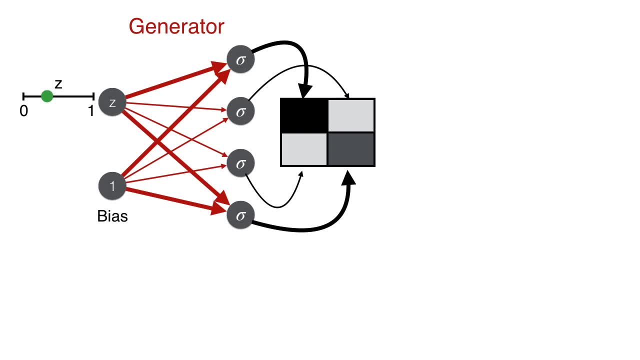 so that gives a small value for this one and therefore our image looks a lot like a diagonal and, given the resolution of the screens in slanted land, that are all two pixels by two pixels and this picture looks uncannily like this resident of slanted land over here. thus we have built a 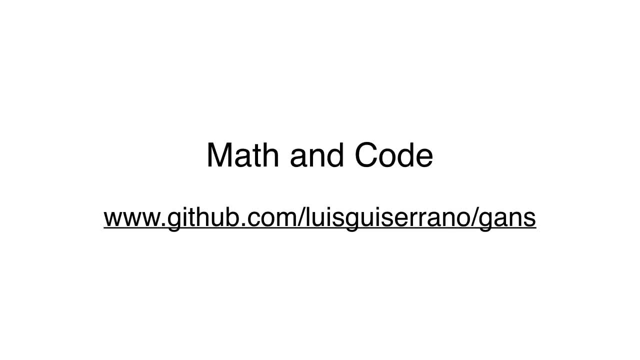 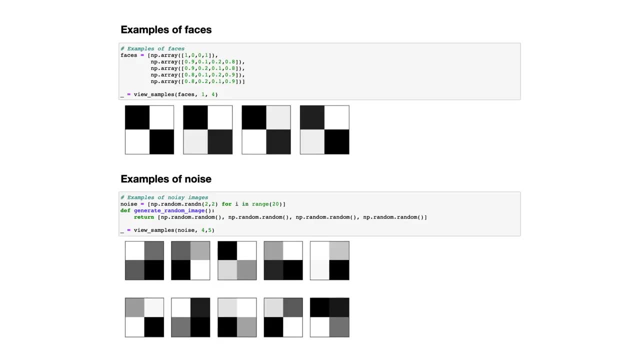 network that generates faces. now, as promised, here's the code for you to sing along to the video. it's in this repo called gans under my github. first we have the faces that we hard code and the random noisy images that we generate that are not necessarily faces. then we also develop the 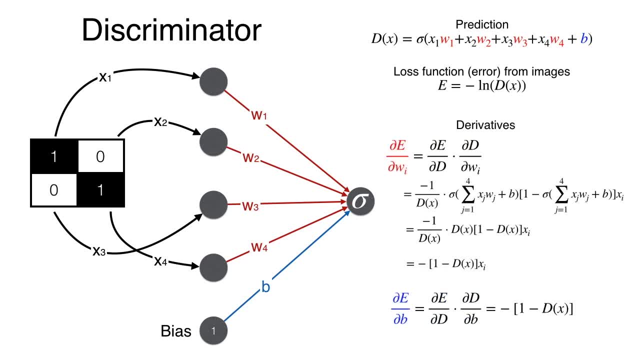 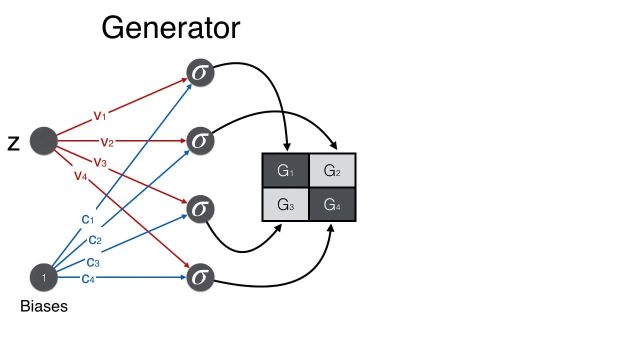 derivatives carefully: for the discriminator based on faces, then for the discriminator based on noisy images, both with respect to the weights and with respect to the biases. these are all coded in this discriminator class. we also work out the derivatives corresponding to the error functions for the generator. again, 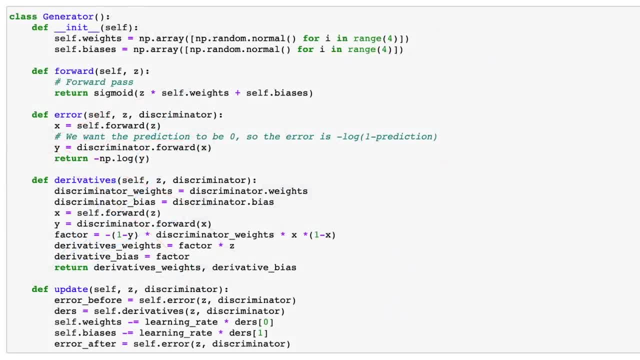 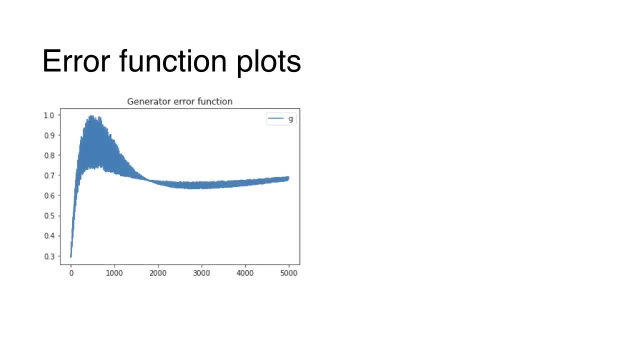 with respect to the weights and the bias, and these are all coded in the generator class. we also have error function plots. we can plot the error function for the generator and the error function for the discriminator. notice that the generator error function goes down and stabilizes, but since the